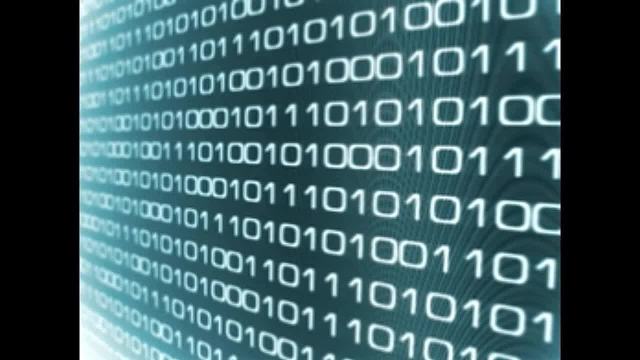 First World War. In the end the world fell into disrepair. The World War II constantly emerged as a world of a few. But in the second world war, with all of the capabilities, the world of games and internautics became more and more complicated. The world started to collapse. The world of games. 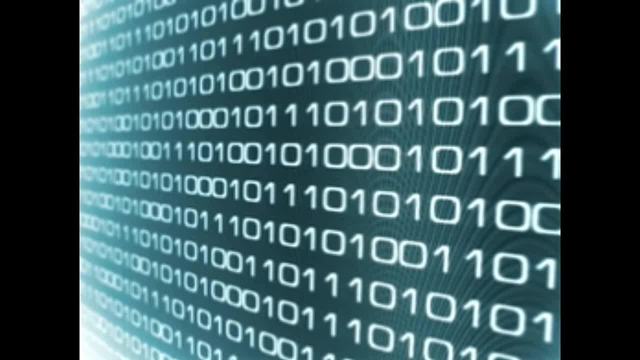 destroyed all accepted conventions, The game changed drastically. Cryptography was rendered practically useless, because there is no technology that is widely available today that prevents the internet service provider from seeing what websites the user visits. Rooting through another server has been used, but this is not a cryptography technique, and 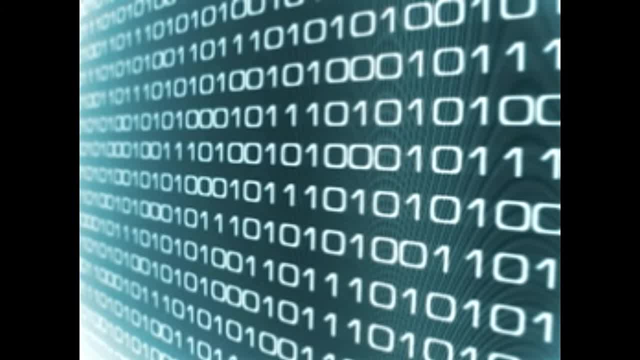 by no means foolproof. Cryptography also has a lot of jargon which scares most first-time readers. Demystifying the jargon is half the battle won for elementary cryptologists. The initial message that is sent is called plaintext. This is then encrypted and converted. 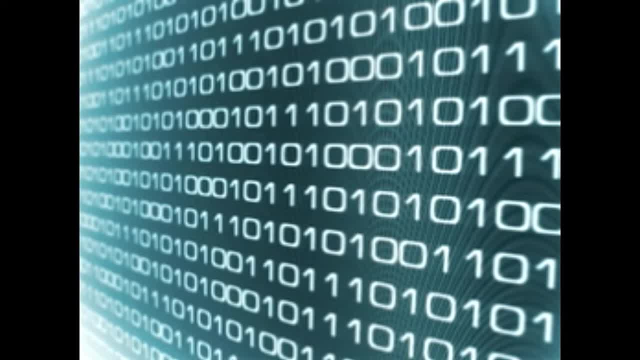 into something called ciphertext. Cryptanalysis is the art of breaking cryptosystems without knowing the decryption key, and cryptology is the study of both cryptography and cryptanalysis. A cryptosystem is usually a whole collection of algorithms. The algorithms are labeled. 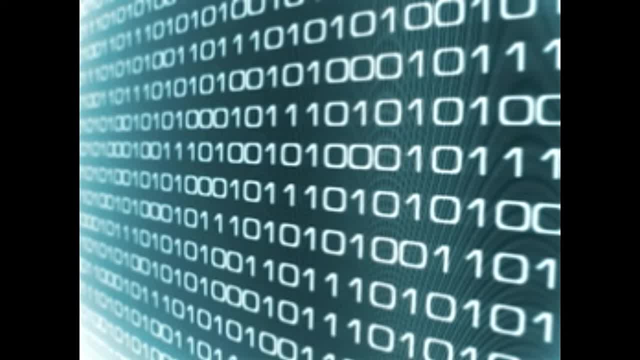 The labels are called keys. In order to decrypt the message, it is important that the proper key is known. When someone gets access to the message without knowing the key, he is called cryptanalyst. The benchmark of great cryptography is that it appears random when confronted with any form of 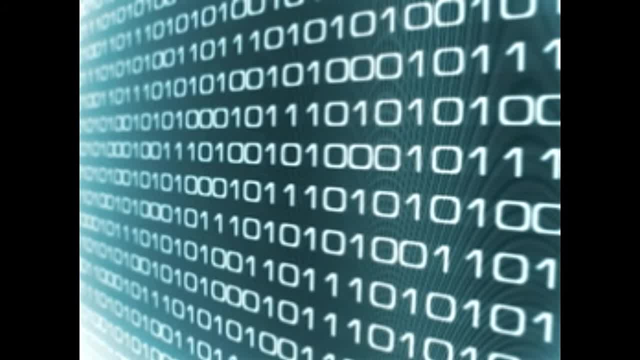 statistical testing. But even when statistics fail to unravel the mystery of cryptography, it is possible that it could be caught out by an ingenious cryptoanalyst. There are two types of key-based encryption algorithms: symmetric and asymmetric algorithms. The difference is that symmetric algorithms use the same key for encryption and decryption. 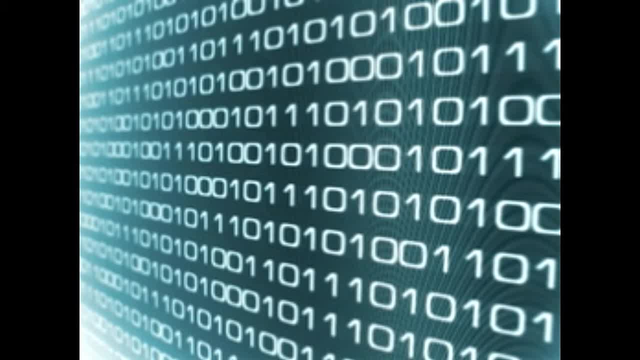 whereas asymmetric algorithms use a different key for encryption and decryption, The decryption key cannot be derived from the encryption key. Symmetric algorithms can be divided into stream ciphers and block ciphers. Stream ciphers can encrypt a single bit of plaintext at a time, whereas blog ciphers can encrypt a number of bits. A digital signature is a small amount of. 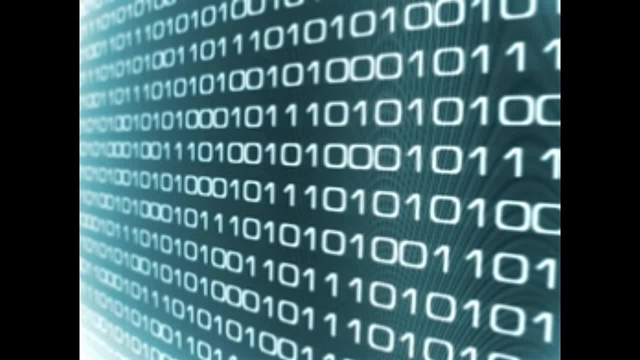 data that was created using some secret key and there is a public key that can be used to verify that the signature was really generated using the corresponding private key. Digital signatures are used to verify that a message really comes from the claimed sender. Cryptography is here to stay. 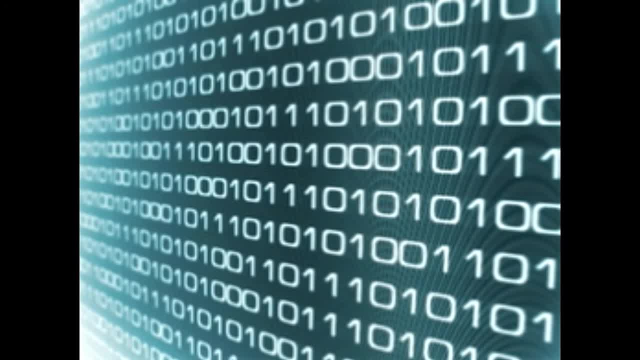 It will evolve to fulfill the ever-increasing security needs of computer users all over the world. The next frontier is the internet. Algorithms have been developed to counter the all-pervasive influence of internet service providers, but they are confined to the realm of. 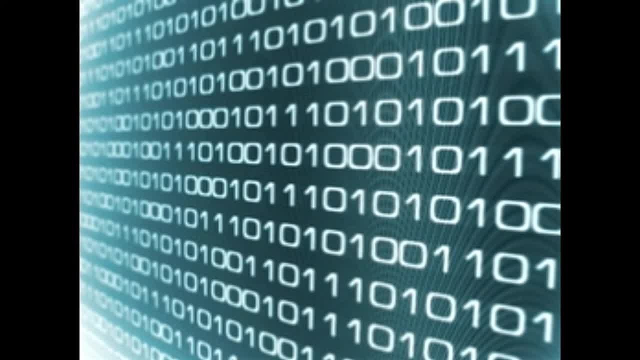 hackers. Cryptography will ensure that this is the norm of tomorrow.